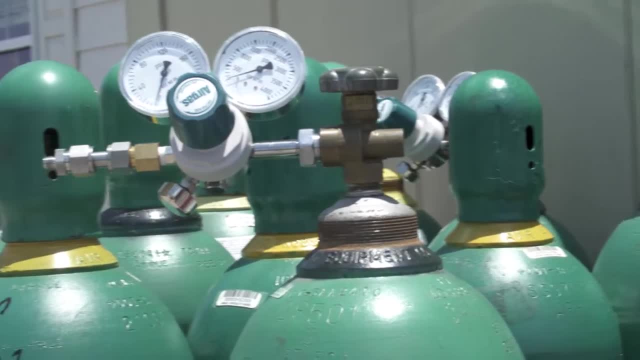 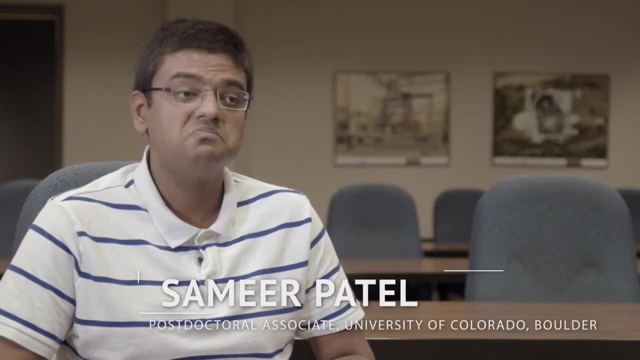 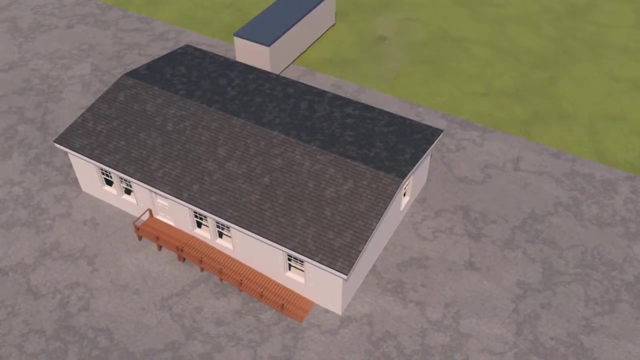 surface chemistry particles, all the air that you breathe. U-Test House at University of Texas Austin is a very unique experimental setup. It's a real house: three-bedroom house, 1,200 square feet. There's a very high density of sophisticated instruments inside the house and the area around the house. 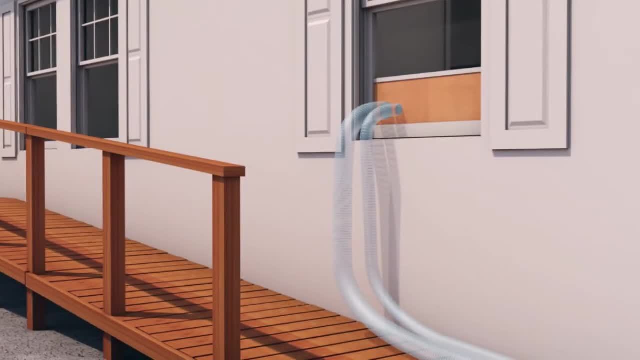 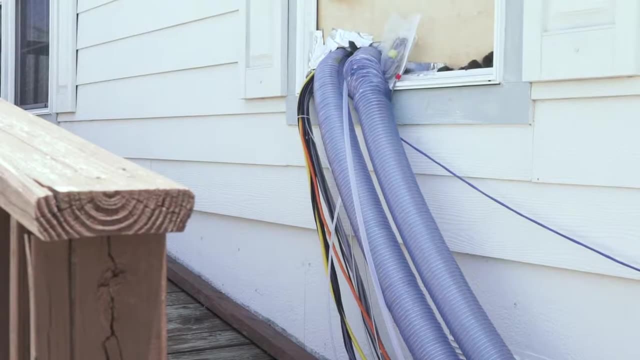 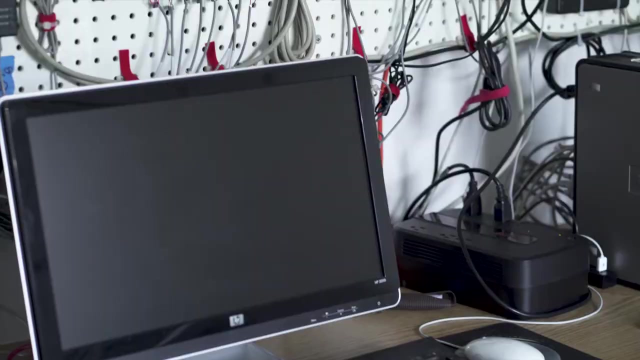 which enables us to simulate real conditions. Unlike permanent houses, this house was built pretty much to be modified and adjusted for various experiments. Cubes and pipes are getting out of the house. You can see the wires are all around to collect air samples. 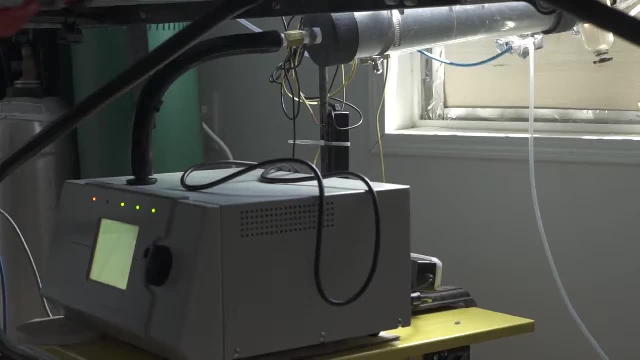 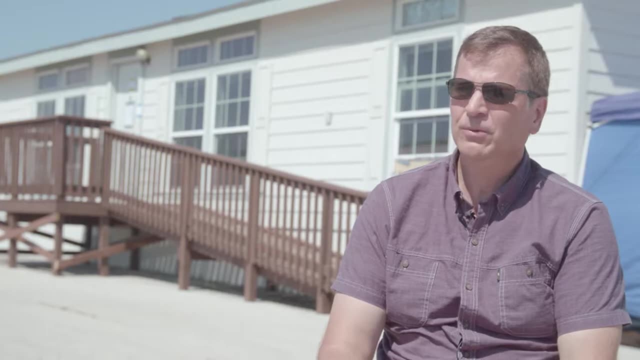 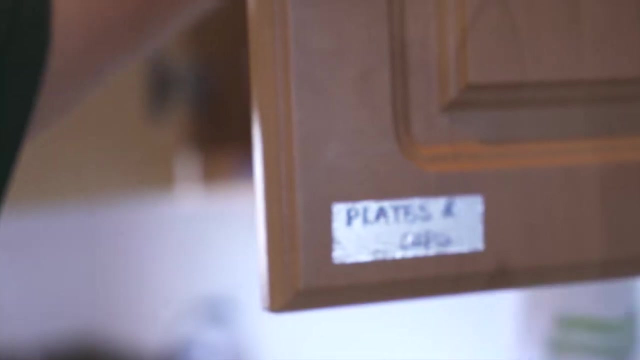 And then it sits outside, So you have ambient conditions and you can look at how the outdoor air quality affects indoor air quality. And that's pretty much what we get with this full-scale test house. So this is the first campaign of its kind and we needed to decide what kind. 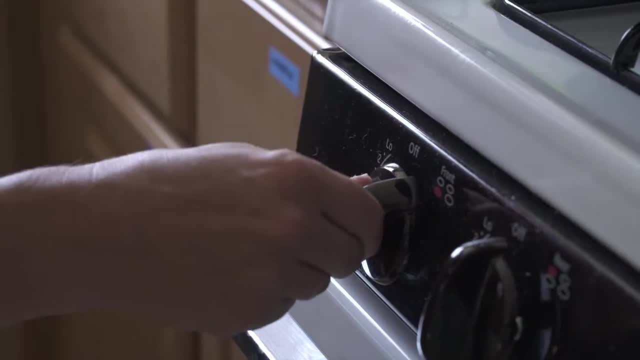 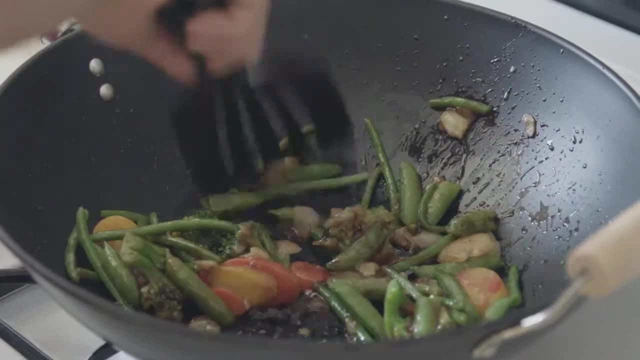 of experiments to run and what level of complication we wanted to get into. So we decided to focus on cooking and cleaning activities. They are both activities that we all engage in, and they can produce emissions of compounds that we're all exposed to. 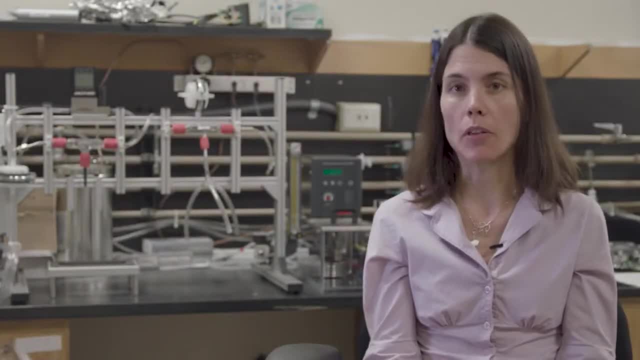 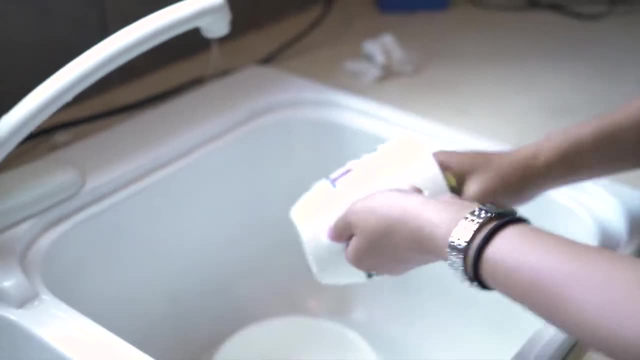 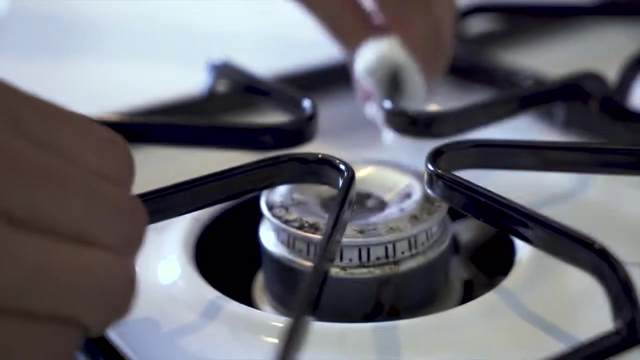 And so there's organic acids and different compounds that are associated with cooking. There's terpene-based cleaners that can result in atmospheric particles when they're oxidized. There's also chlorine-containing compounds in chlorine-containing disinfectant solutions that we are looking at. 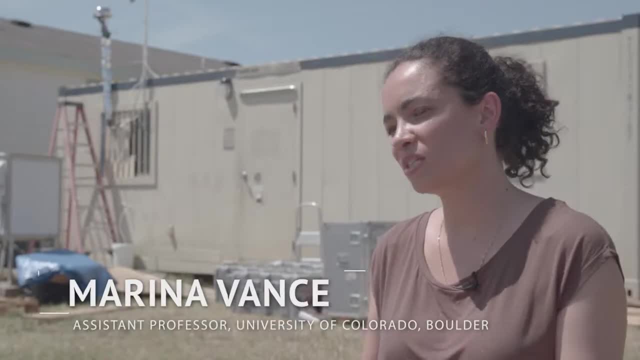 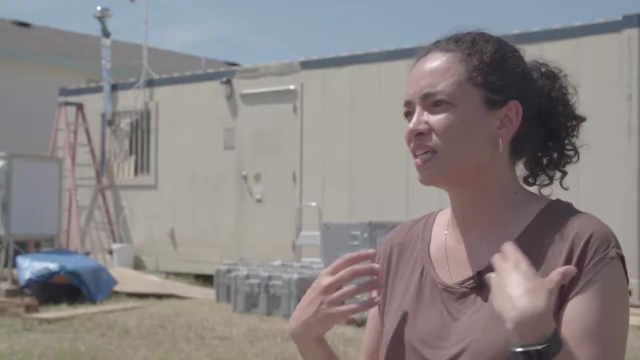 We are also looking at human occupancy. What we're measuring is basically the human fingerprint, and that includes reaction products. things that are coming off of your skin, things that are naturally coming from your body- For example, our human sweat- have lactic acid in it. 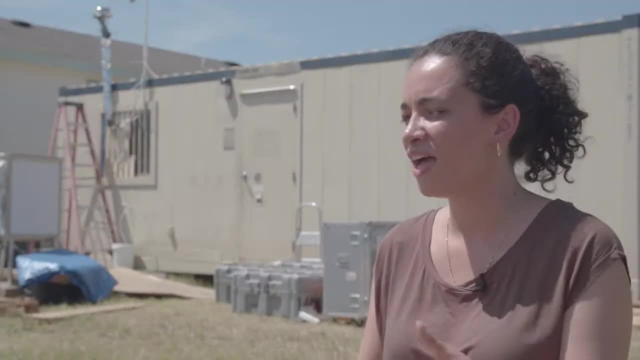 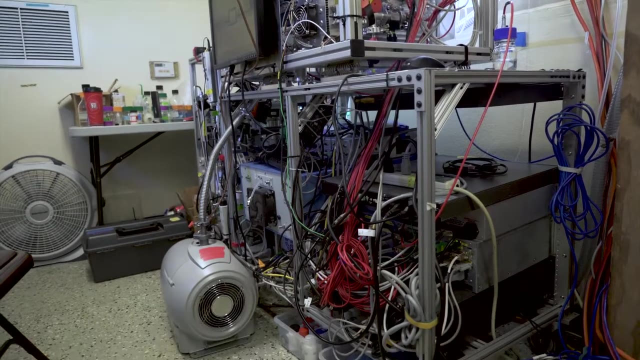 So we're trying to see what kind of reactions can happen later on after these things are emitted into the environment. The research teams associated with Home Chem are measuring a wide spectrum of different pollutants. Historically in the past, we would collect air samples. 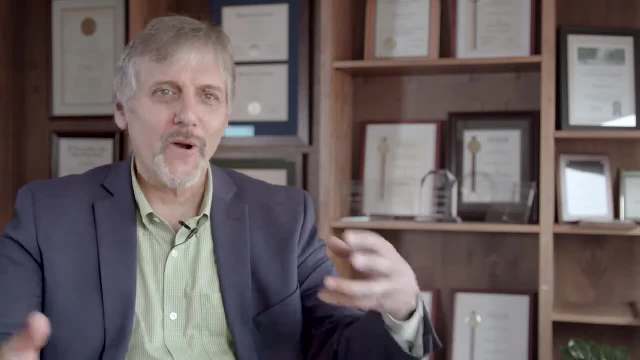 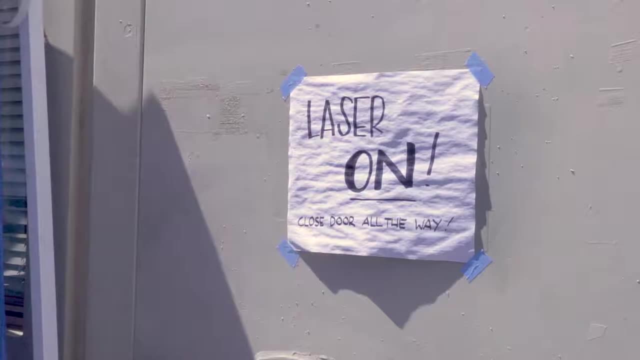 over many, many hours and then bring the samples to the laboratory and it would take hours to analyze what was on them. These instruments are so sophisticated- they can measure what's in a room in real time. There's a group from Indiana University.